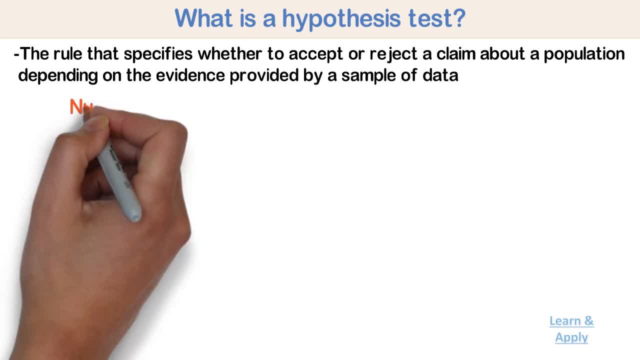 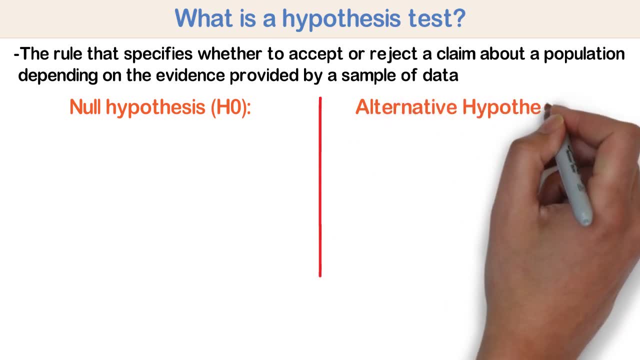 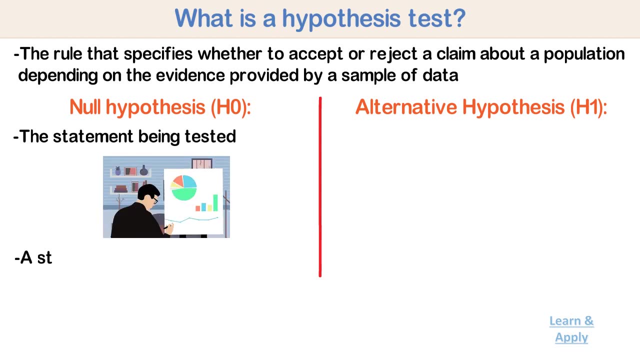 by a sample of data. A hypothesis test examines two opposing hypotheses about a population: the null hypothesis and the alternative hypothesis. as seen in the last video, The null hypothesis is the statement being tested Usually. the null hypothesis is the statement of no effect or null. 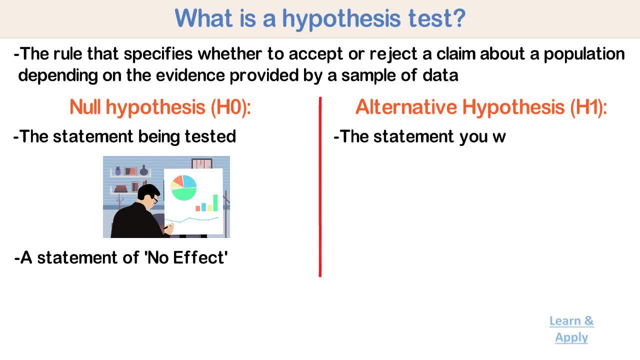 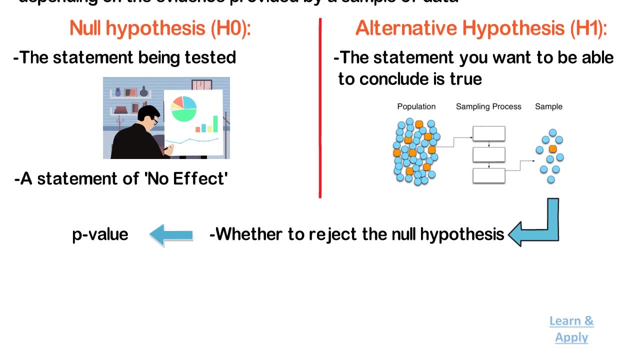 The alternative hypothesis is the statement you want to be able to conclude is true based on the evidence provided by the sample data. Based on the sample data, the test determines whether to reject the null hypothesis. You use a p-value to make this determination. 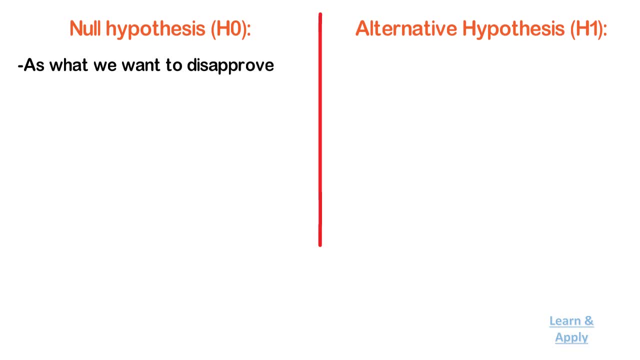 The null hypothesis appears what we want to disapprove, Because we fixed the significance level to be small before the analysis. usually a value of 0.05 works well when we reject the null hypothesis, So that's the reason why a null hypothesis test is valid here. 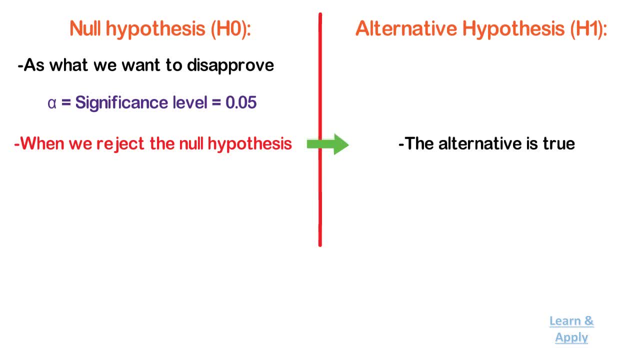 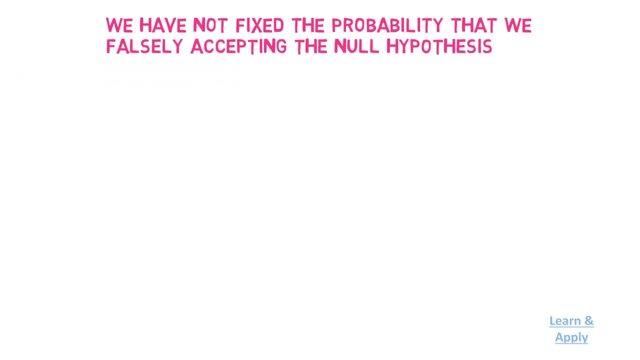 The null hypothesis test anyway has a statistical proof that the alternative is true. Conversely, if we fail to reject the null hypothesis, we do not have a statistical proof that the null hypothesis is true. This is because we have not fixed the probability that we are falsely accepting a null hypothesis to be small. 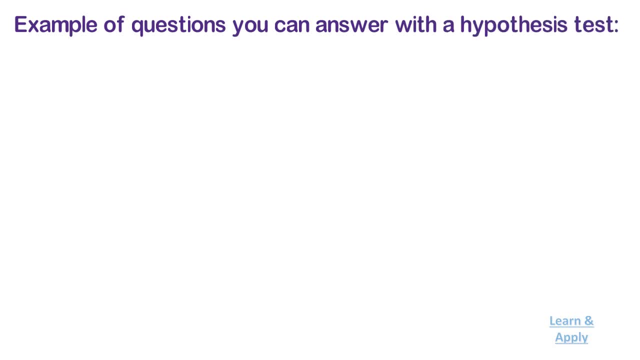 Example of questions you can answer with a hypothesis test includes: Does the average marks in science of Class 9 students of the ABC school differed by 85?? does the mean height of students differed from 66 inches? is the standard division for height of students equal to or less than 5 inches and are the proportion of passing a class 9 students? 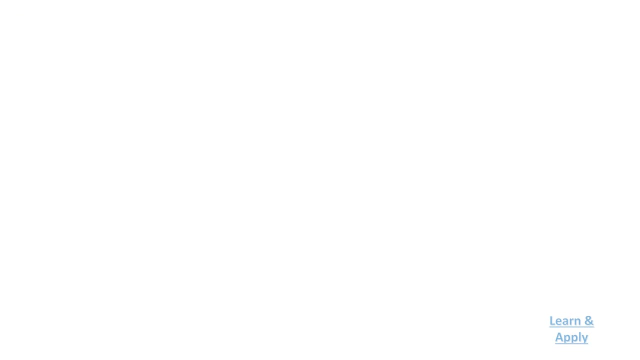 significantly higher than the proportion of class 8 students. example of performing a basic hypothesis test. this is a general procedure to conduct a hypothesis test. we will see detailed procedure for each type of test, including sample size, data consideration, with the help of practical example, in future videos. let's see this procedure with an example. an economics wants to determine. 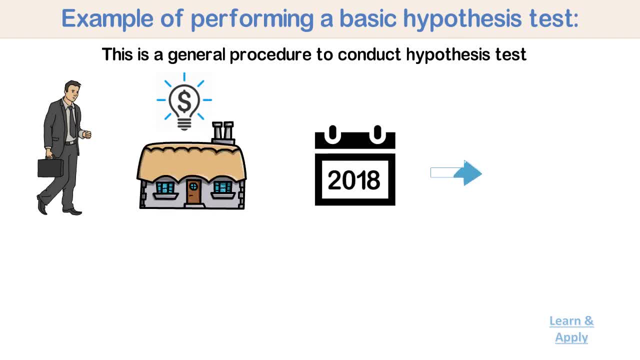 whether the monthly energy cost for families has changed from the previous year when the mean cost per month was 200 dollars. the economics follows the basic steps for doing a hypothesis test. one specify the hypothesis first. the economics formulates the hypothesis. the null hypothesis is monthly energy cost families. 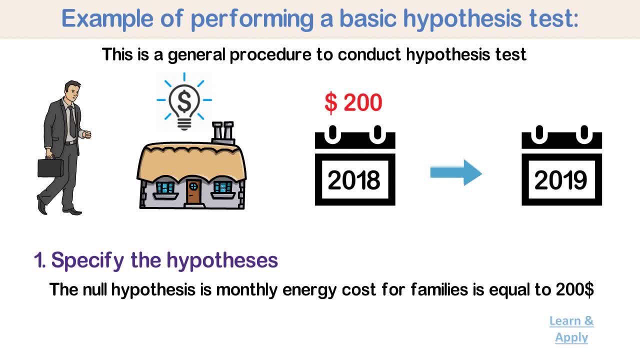 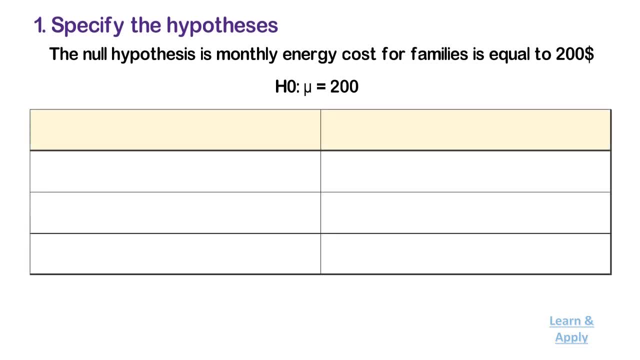 is equal to 200 dollars. formally this is written as: h0 colon mu is equal to 200, then the economics selects from the following alternative hypothesis condition to test: the population mean is less than the target and the alternative hypothesis is: one-sided mu is less than 200. second, the population mean is greater than the target and alternative hypothesis is: 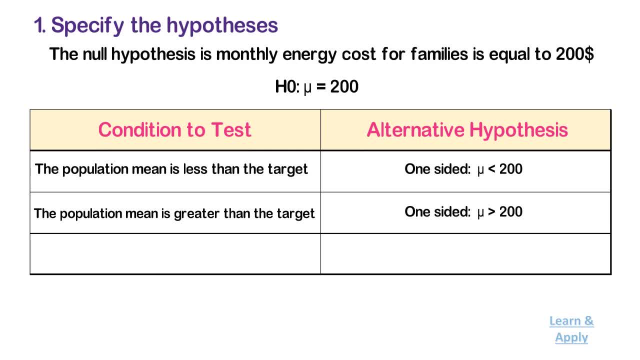 one-sided mu is greater than 200 and third, the population mean differs from the target and alternative hypothesis is two-sided mu is not equal to 200 because they need to ensure that the monthly energy cost for families has changed from the previous year. the economics selects the two-sided. 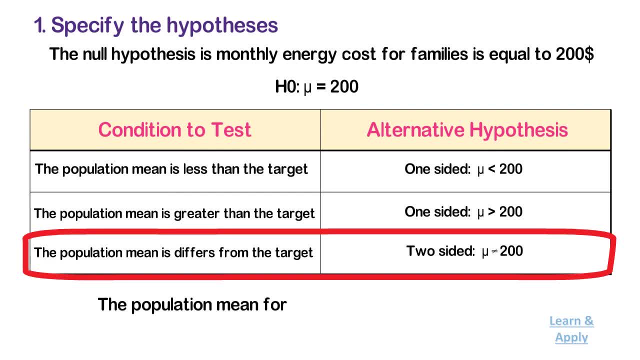 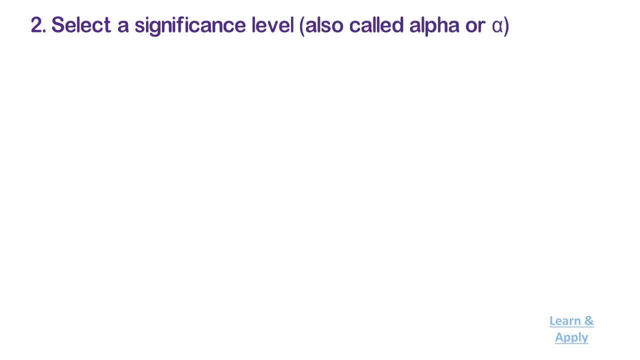 alternative hypothesis. we stress that the population mean for energy cost is not equal to 200. formally this is written as: h1. colon mu is not equal to 200. colon mu is not equal to two hundred. to select a significance, Apps Nada Alpha. The economics use a power and sample size calculation to determine how many families 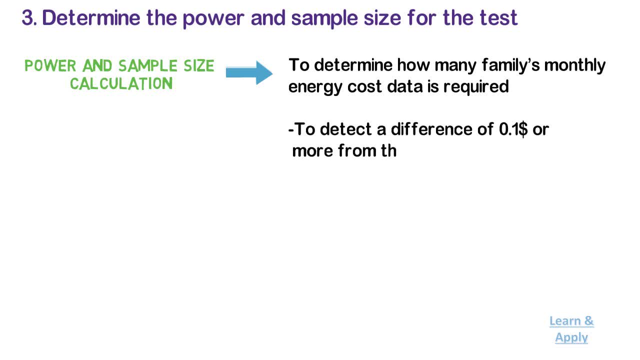 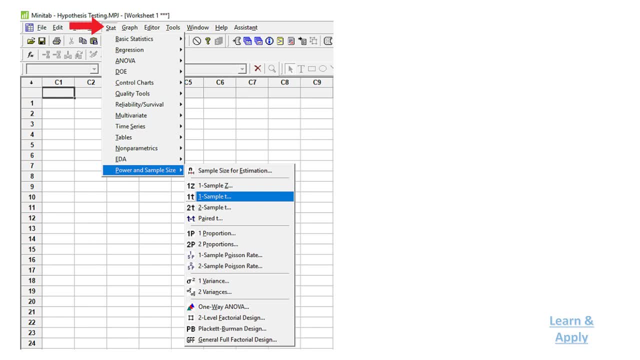 monthly energy cost. data is required to measure to have a good chance of detecting a difference or more from the target. To find the sample size, he followed the procedure: 1. Select stat power and sample size and then 1 sample t-test. 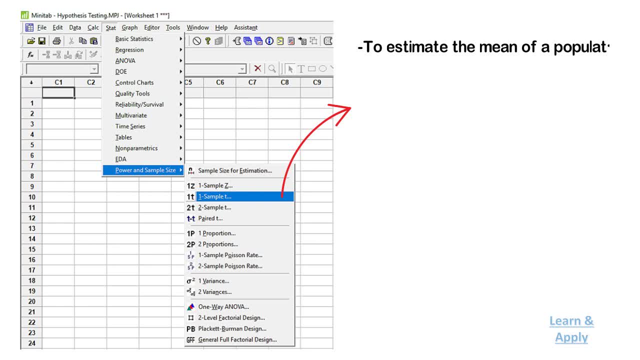 He used a 1 sample t-test because it is used to estimate the mean of population and to compare it to a target value or a reference value when you do not know the standard deviation of the population. 2. Specify the value for differences as 0.1.. 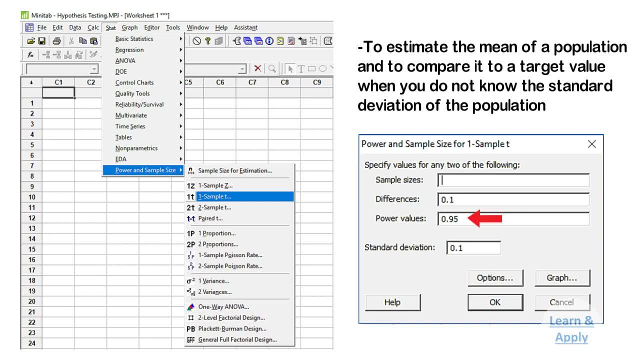 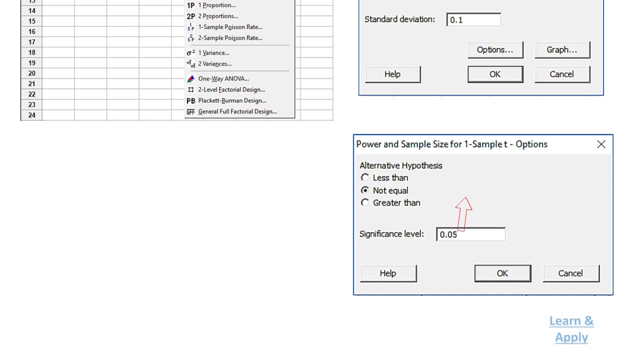 3. In power values: enter 0.95.. 4. In standard deviation: enter the sample standard deviation. Let's say it is 0.1.. 5. Click options. 6. In alternative hypothesis: select not equal. 7. Click ok in each dialog box to get the